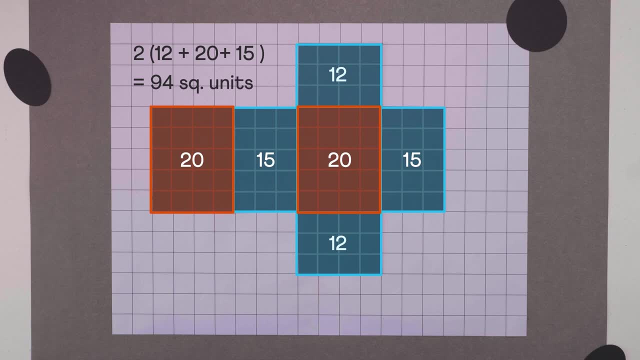 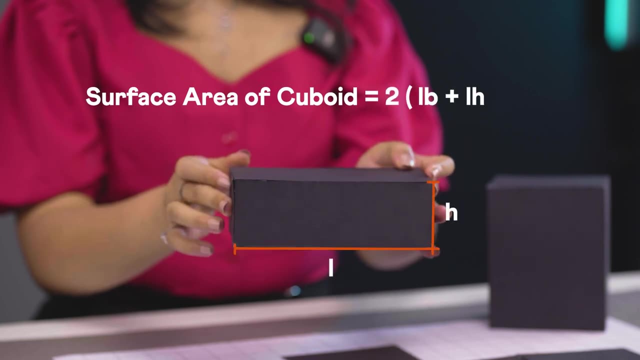 plus 20 plus 15, that's 94 square units. Similarly, we can find the surface area of any cuboid as twice of length times breadth plus length times height plus breadth times height. A cuboid is a special kind of 3D shape called a prism. 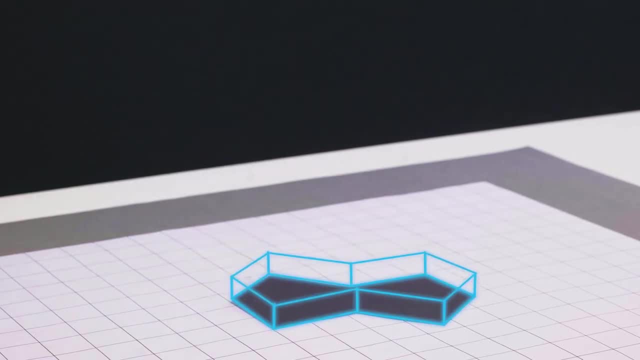 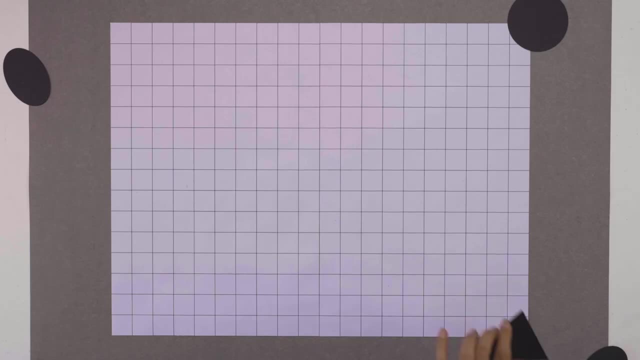 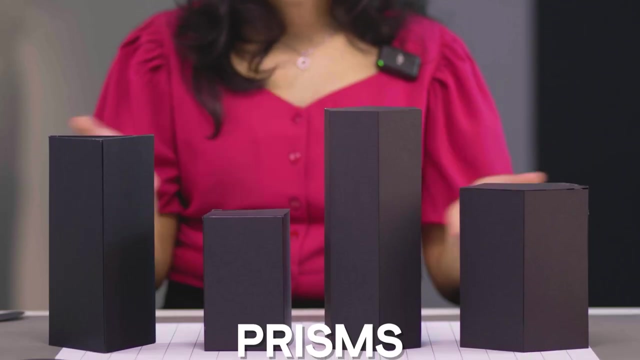 What's a prism exactly? Take any shape. now imagine it extending perpendicularly up from the sheet of paper. that's an upright prism. For example, take a triangle, and that's a triangular prism, Pentagonal prism, hexagonal prism, and all these are just prisms. 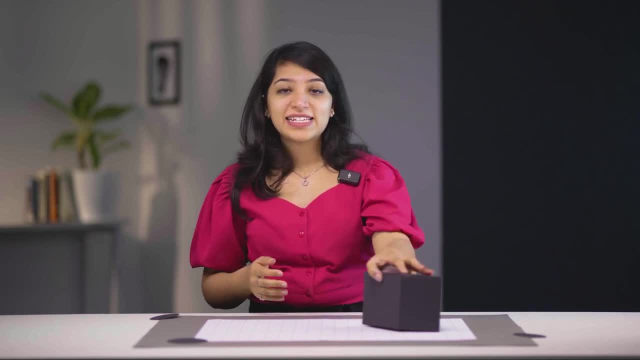 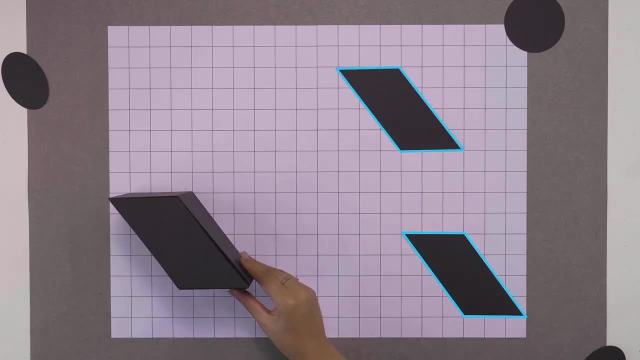 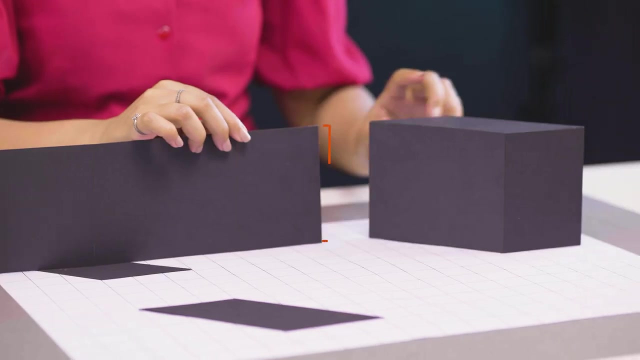 Can we arrive at a formula to find their areas? Let's unfold this prism with a parallelogram base and see how it looks. We get 2 equal parallelograms from its top and bottom. All these faces are rectangles. Together they form a bigger rectangle. Its breadth equals the height. 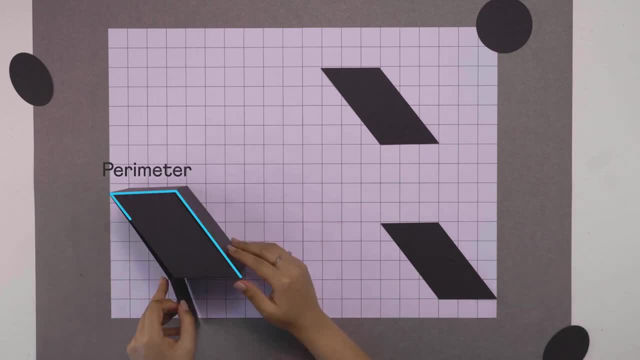 of the prism and its length equals the perimeter of the parallelogram. that is, 3 plus 5 plus 3 plus 5 or 16 units. So the area of this rectangle is 3.5 plus 3 plus 5 or 16 units. 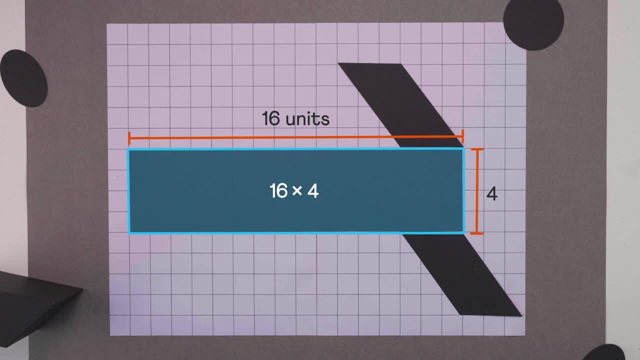 So the area of this rectangle is 4.5 plus 3 plus 5 or 16 units. So the area of this rectangle is is 16 times 4 or 64 square units. The area of each parallelogram is base times height. 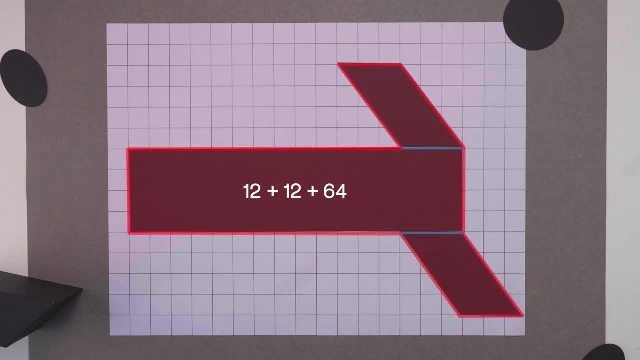 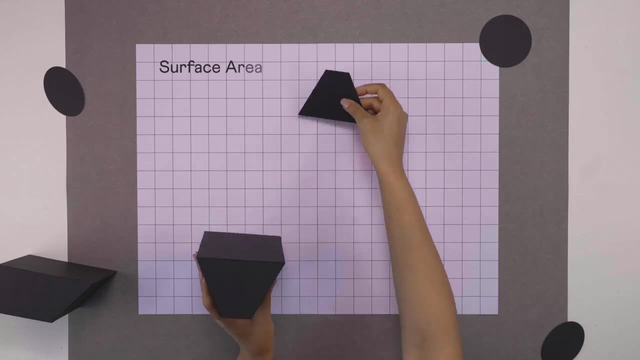 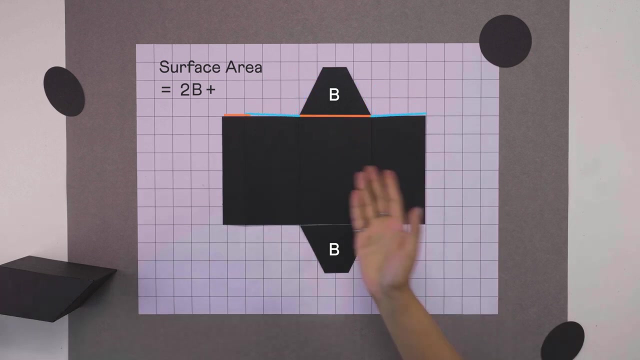 that's 12 square units. Adding these areas gives the surface area of the prism. that is 88 square units. We can find the surface area of any prism. similarly, It's twice the area of the base plus the area of the unfolded rectangle which is the product of the base. 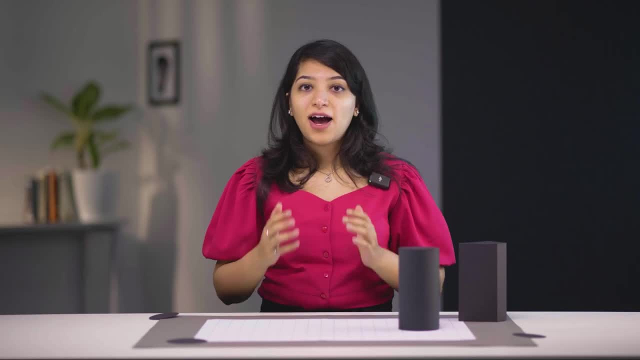 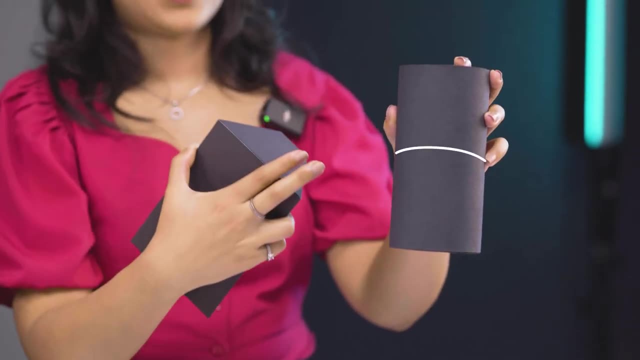 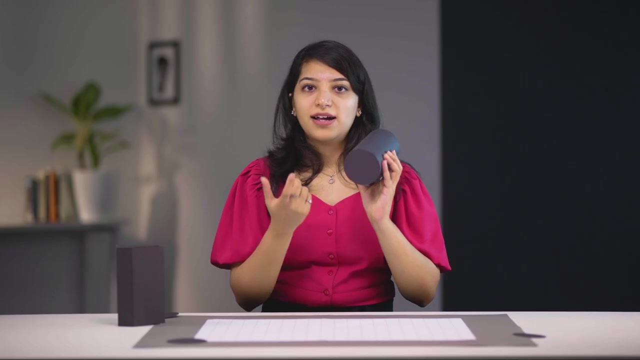 perimeter and the height of the prism. How about this? shape a cylinder. Unlike the flat surfaces of a prism, this one has a curved surface, but we can think about its surface area in a similar manner. The areas of its top and bottom are circles, which is pi? r squared. but what about? 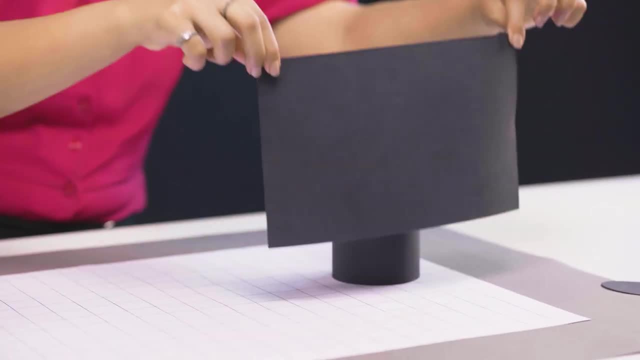 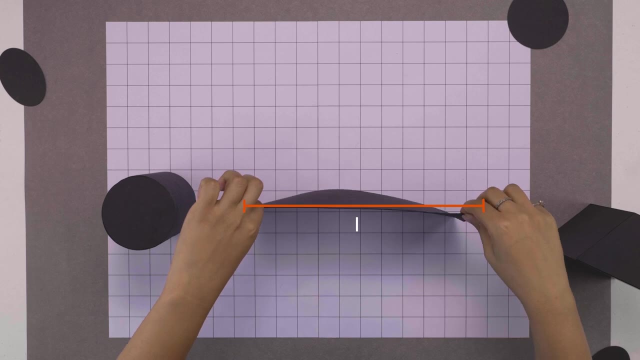 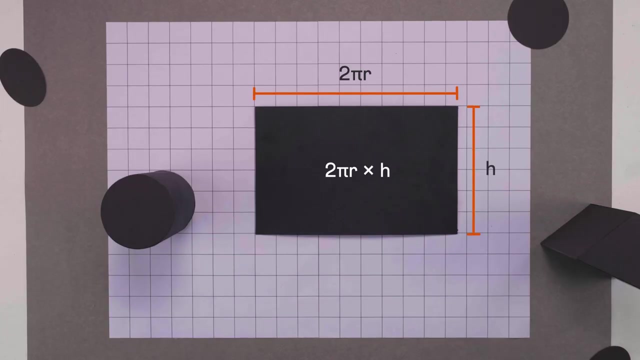 this curved surface. If we open it up it turns into a rectangle. Its width must equal the height of the cylinder and its length equals the perimeter of the circle. that's 2 pi r. so its area is 2 pi r times h. So the total surface area of any cylinder is the area of the two circles plus the curved.